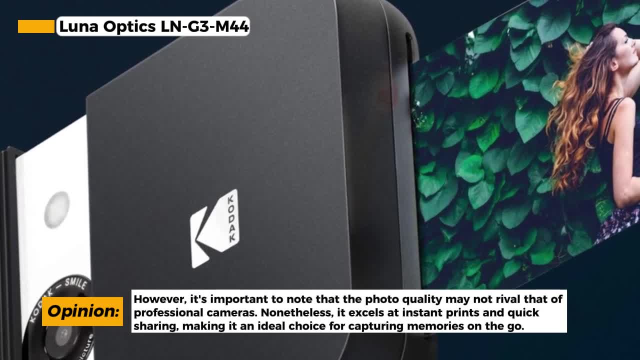 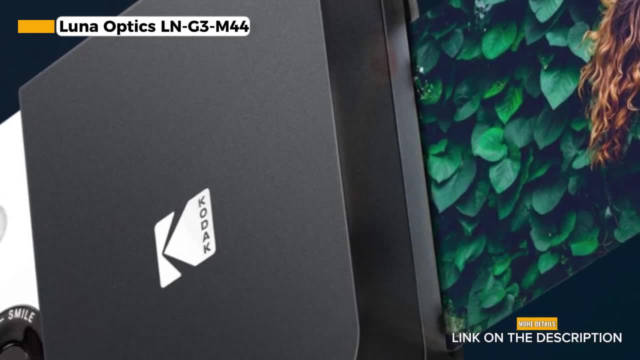 personal photo booth on the go, which is sure to bring smiles to your face. However, it's important to note that the photo quality might not match that of professional cameras. It's designed for instant prints and quick sharing, so, while it might not be, 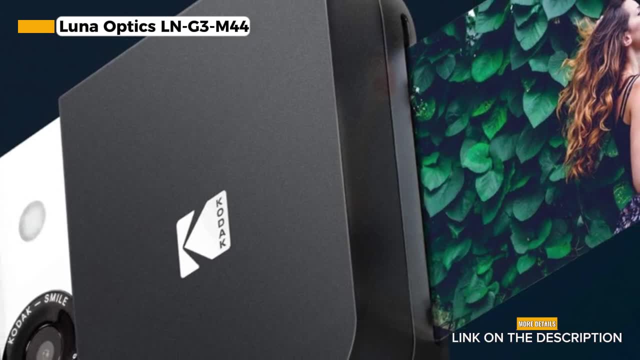 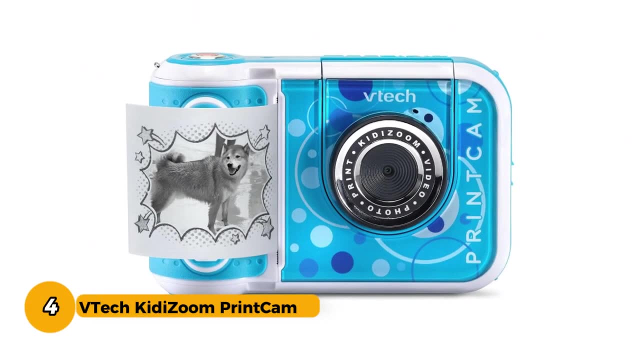 ideal for high-quality photography. it's perfect for capturing memories on the fly. Number 4. VTEC Kidizoom Print Cam. The VTEC Kidizoom Print Cam is not just a camera. it's a world of creativity for your child. 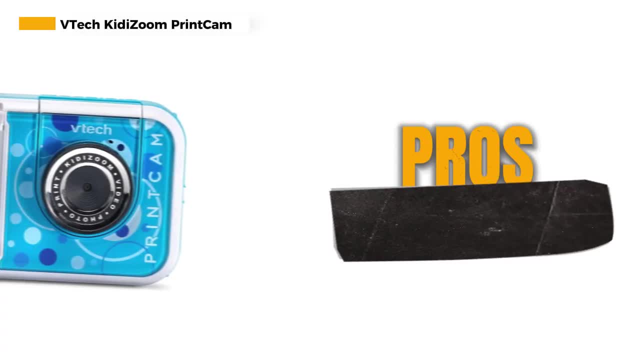 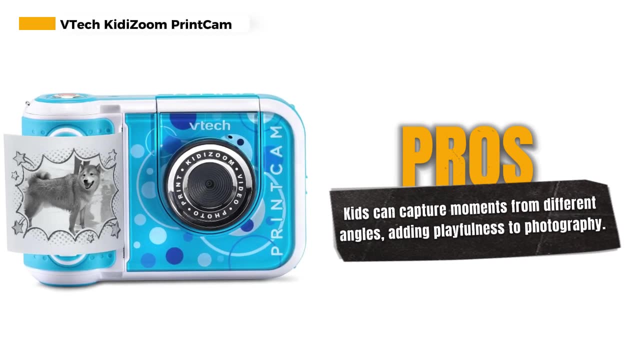 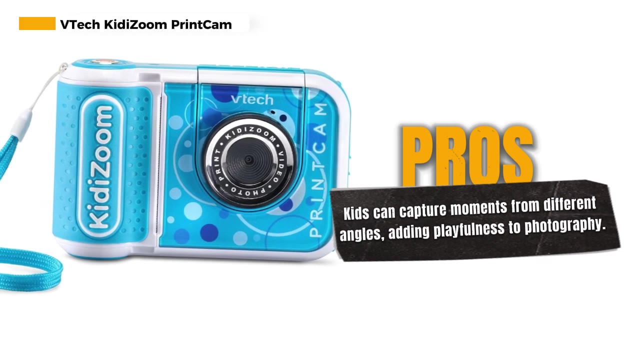 This instant camera is designed to inspire young minds, making photography a fun and interactive experience. One of the coolest features of the Kidizoom Print Cam is its flip camera lens. It's not just practical, it's fun to use. Kids can capture moments from different angles, adding a 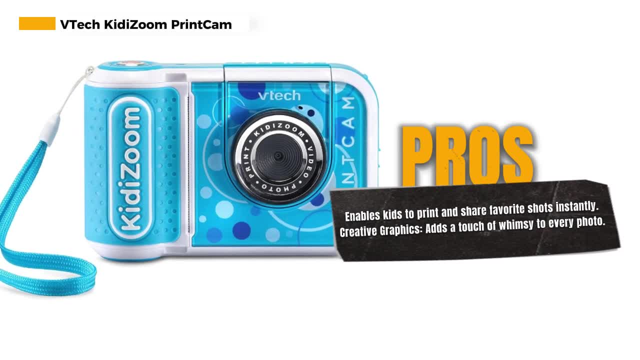 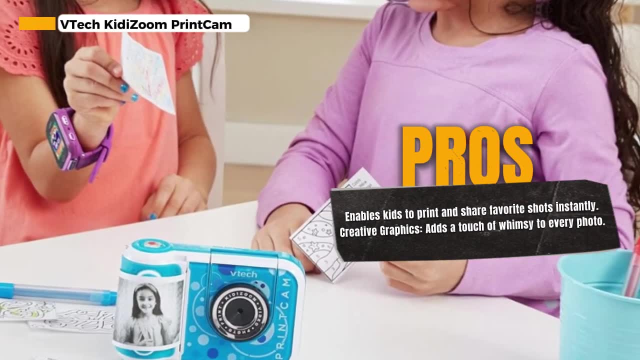 playful twist to their photography. It's a great way to capture moments from different angles, adding a sense of humor. adding a sense of humor, adding a sense of happiness to their life. Affordable photo prints make this camera a parent's dream. It allows kids to print and share their favorite shots, bringing their creations to life in an 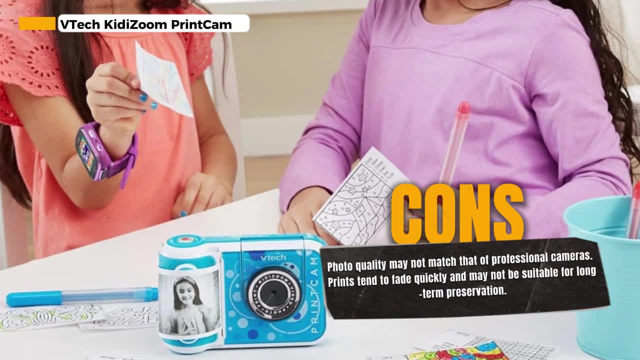 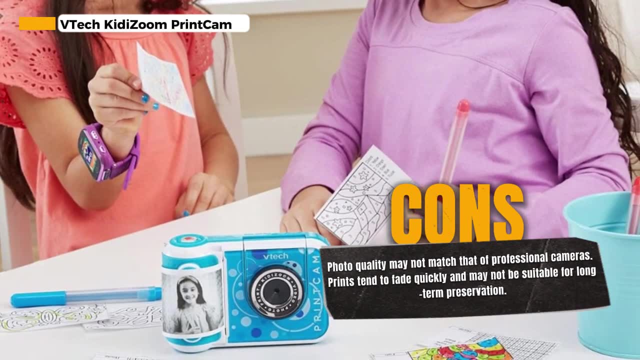 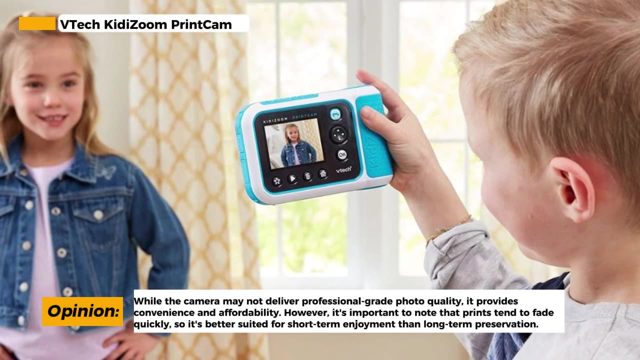 instant Plus. the fun, creative graphics add a touch of whimsy to every photo. However, there are a couple of downsides to consider. Some users have reported that the photo quality can be sub-par. While it might not match the quality of professional cameras, it's a trade-off. for the convenience and affordability. However, it's not just for good use. Some users have reported that the photo quality can be sub-par. While it might not match the quality of professional cameras, it's a trade-off for the convenience and affordability. 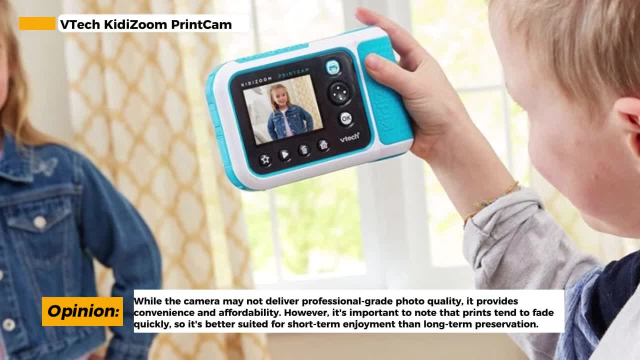 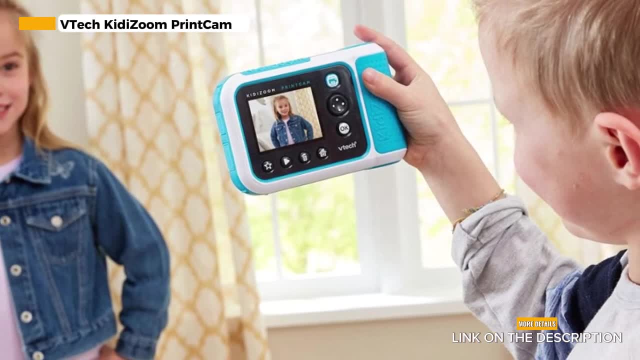 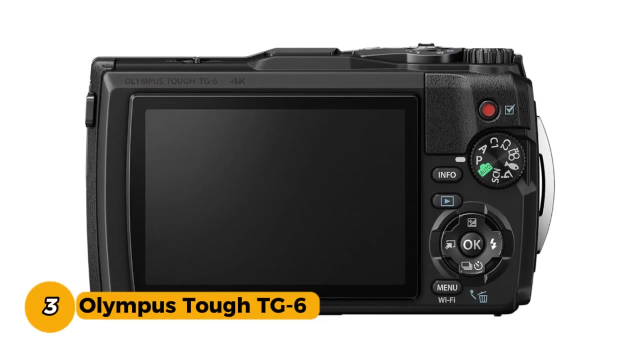 Another point to note is that the prints from the Kidizoom print cam tend to fade quickly. While they're great for short-term enjoyment, they might not be the best choice for preserving memories over a long time. Number 3. Olympus Tough TG6.. The Olympus Tough TG6 is your trusted companion for capturing. 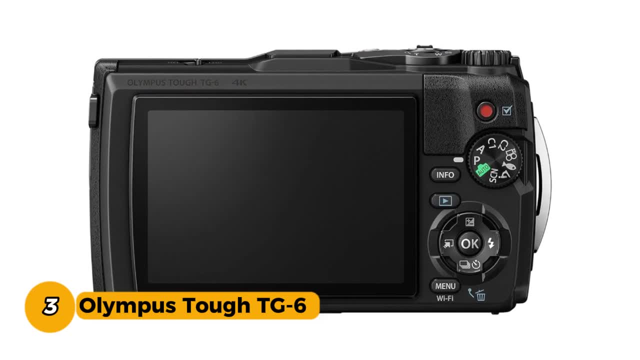 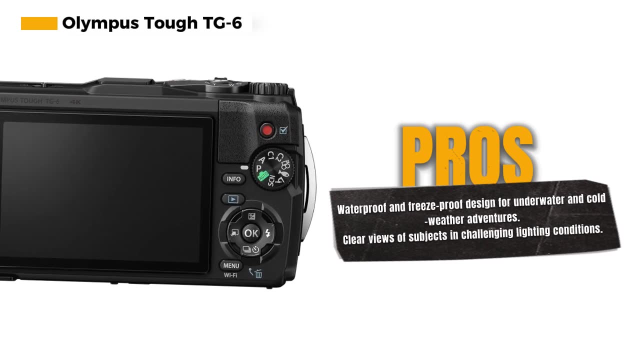 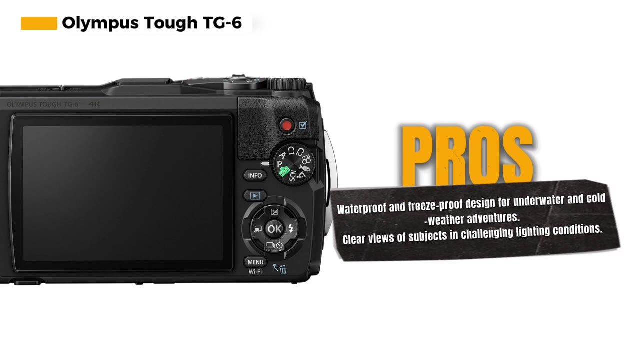 incredible moments in extreme conditions. This underwater camera is not just tough, it's outstanding in every aspect, ensuring your memories are as vivid as your experiences. Designed for adventure, the TG6 is waterproof and freeze-proof, allowing you to explore both beneath the waves and in frigid temperatures. It's a camera that can keep up with your most. 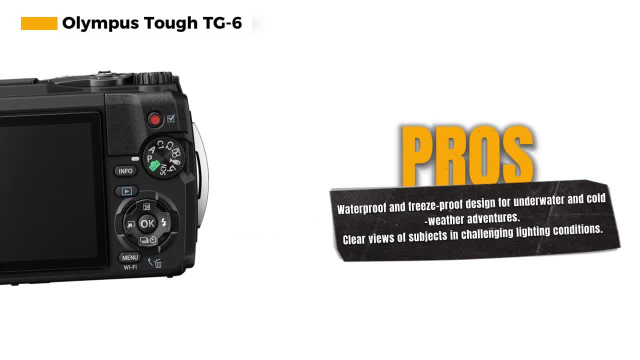 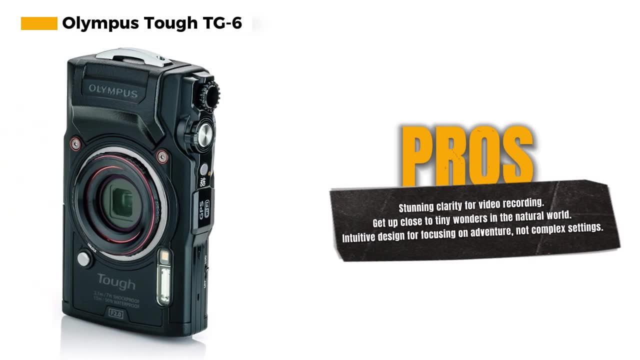 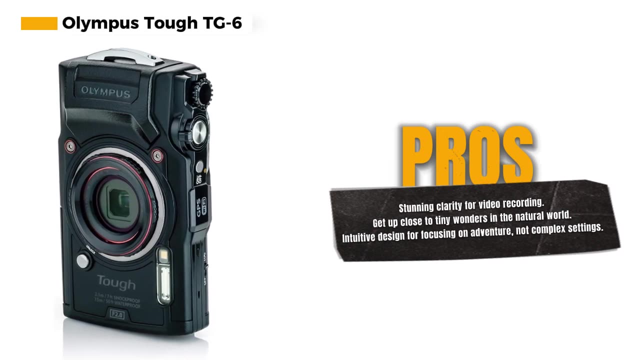 daring escapades. One of the standout features of the TG6 is its high-resolution and bright display. This ensures that you'll always have a clear view of your subjects, even in challenging lighting. Whether you're shooting underwater or in low-light environments, this camera delivers. 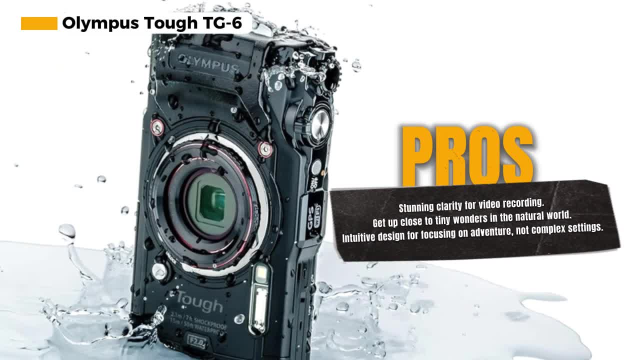 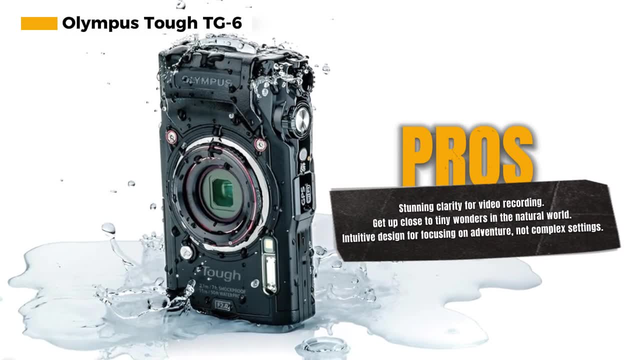 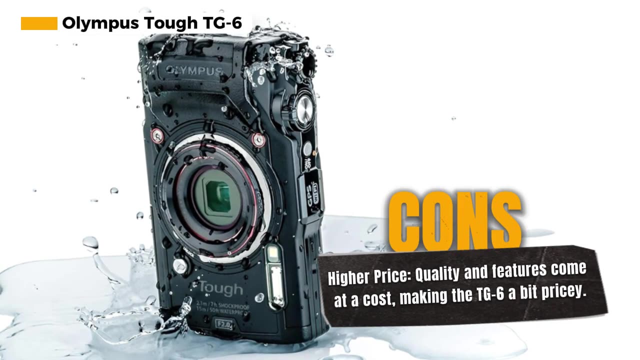 And let's talk about the 4K video capability. It's not just video, it's a visual masterpiece. With 4K video, your adventures come to life and you can relive them with stunning clarity. The 44x macro shooting feature lets you get up close to tiny wonders in the natural world. 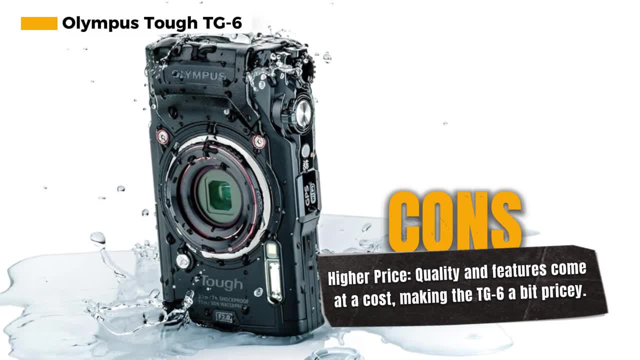 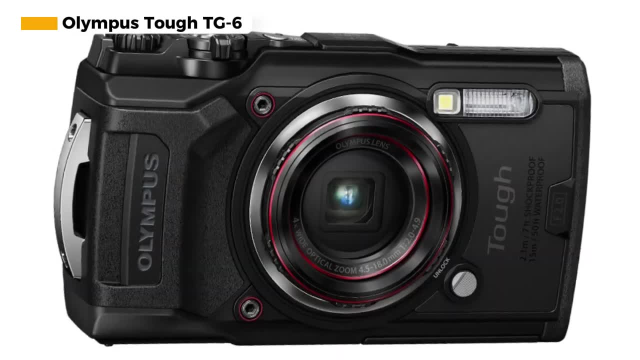 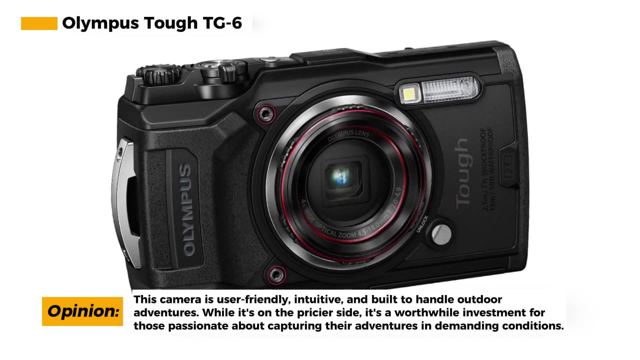 adding a whole new dimension to your photography. The TG6 is not just about functionality: it's user-friendly too. It's an intuitive camera so you can focus on your adventure without fumbling with complex settings. The durable build ensures it can handle the rough and tumble of outdoor life. 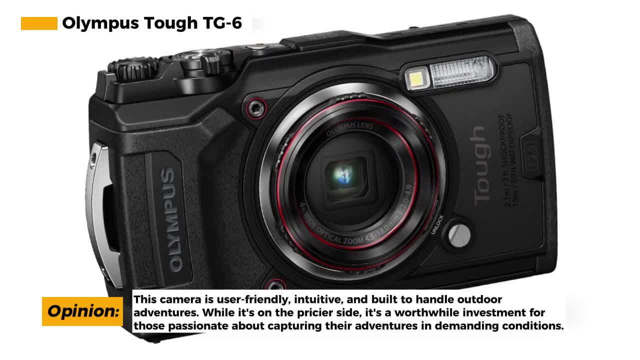 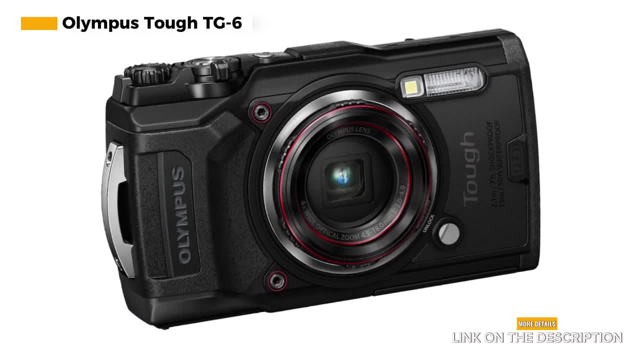 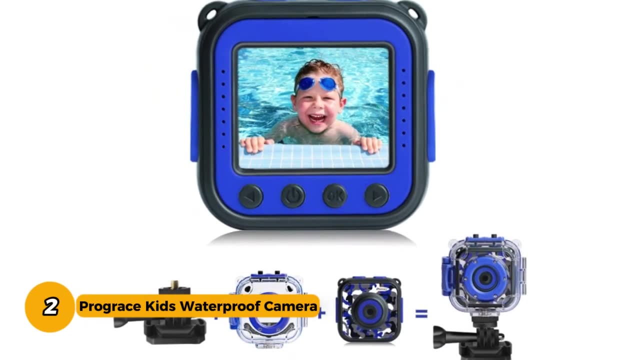 However, it's important to mention that quality comes at a price. The TG6 is a bit on the costly side, but it's a worthwhile investment for anyone who loves capturing their adventures in extreme conditions. Number 2, Prograce Kids Waterproof Camera. The Prograce Kids Waterproof Camera is more 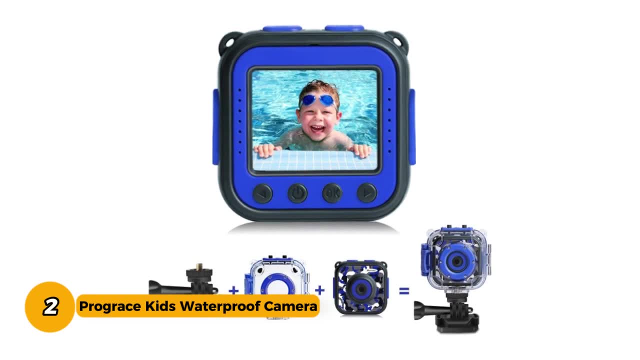 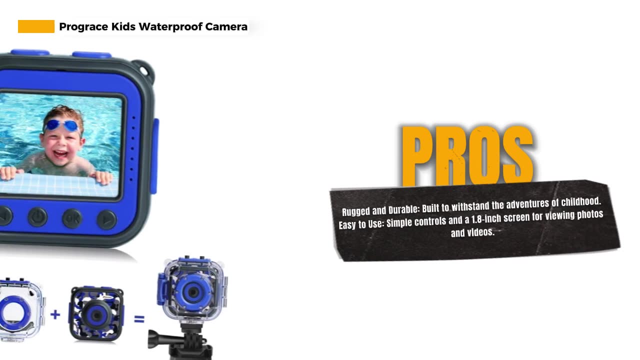 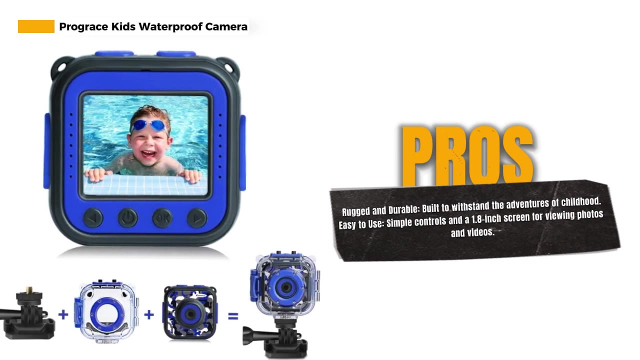 than just a camera. it's a gateway to endless adventures for your little ones. Designed with kids in mind, this action video digital camera is a perfect companion for budding explorers. This rugged camera is built to withstand the adventures of childhood. It's durable and can handle a few bumps and splashes. 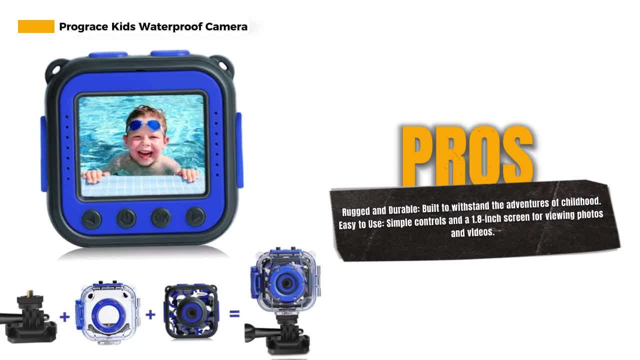 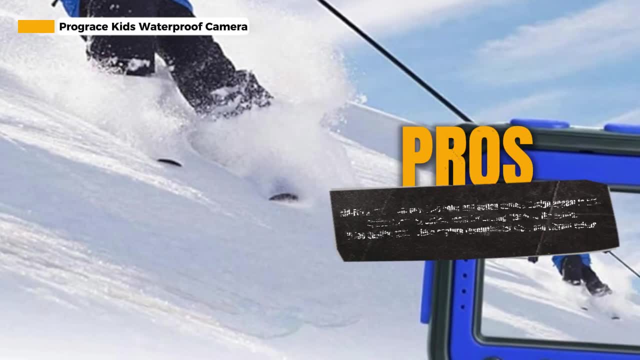 making it a great camera to use when you're out and about. The Prograce Kids Waterproof Camera is designed to be fun to use and it truly lives up to that promise. With a 1.8-inch screen, kids can view their photos and videos, and the simple controls. 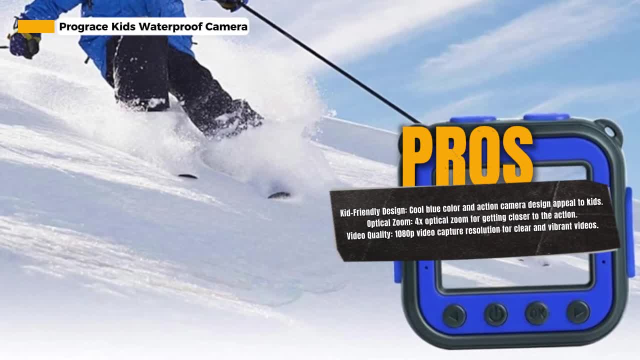 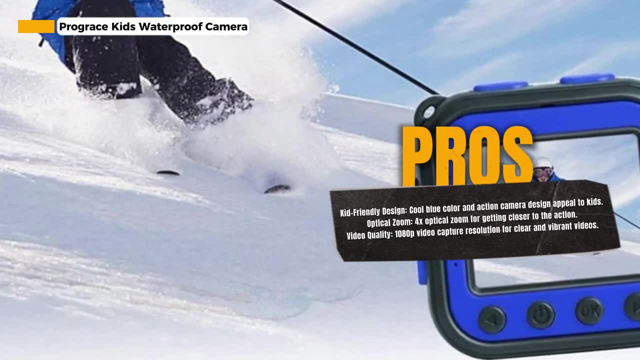 make it easy for them to take pictures and record videos without any hassle. The cool blue color and action camera design make it even more appealing to kids. It's not just a camera, it's a fashion statement for the young adventurers. The Prograce Kids Waterproof Camera is a great camera to use. 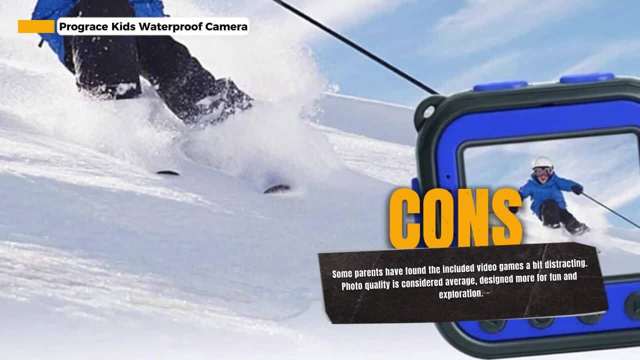 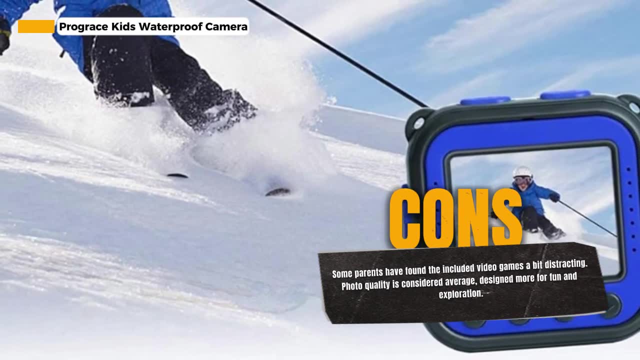 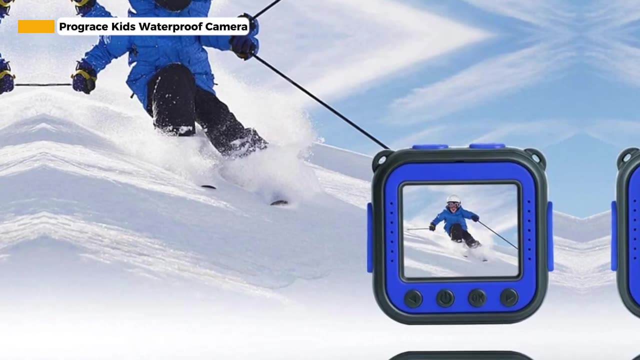 when they're out and about. With an optical zoom of 4x, kids can get closer to the action, whether it's wildlife, friends or the sights of their adventures. The camera also boasts a video capture resolution of 1080p, ensuring that their videos are clear and vibrant. Now let's address 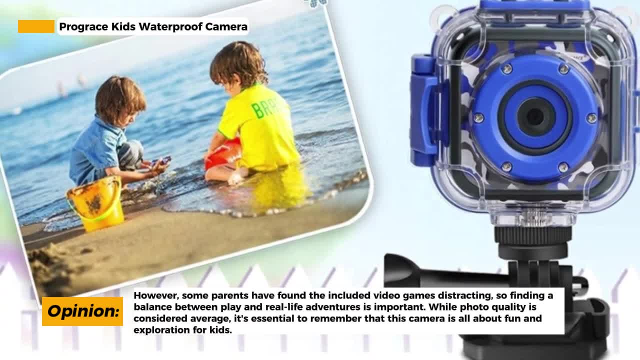 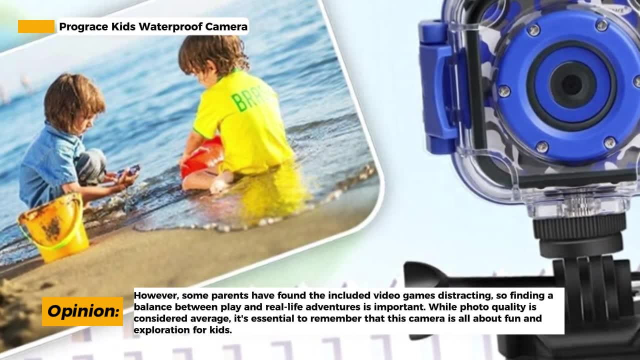 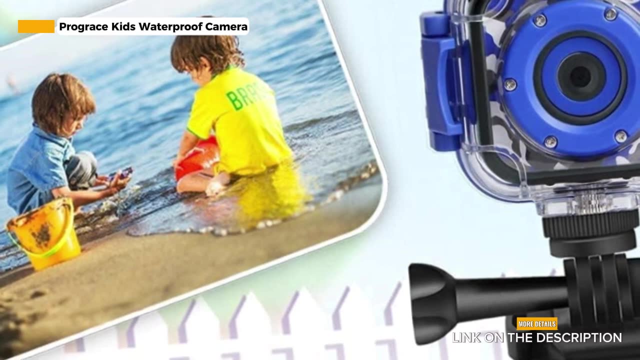 the drawbacks. Some parents have reported that the video games included with the camera can be a bit distracting. While they can be fun, it's essential to find the right balance between play and capturing real-life adventures. Additionally, the photo quality is considered SOSO. It's important. 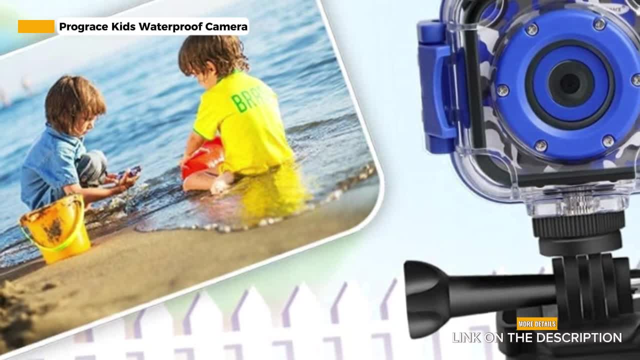 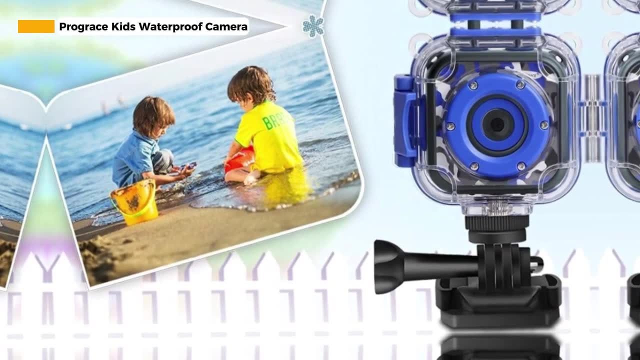 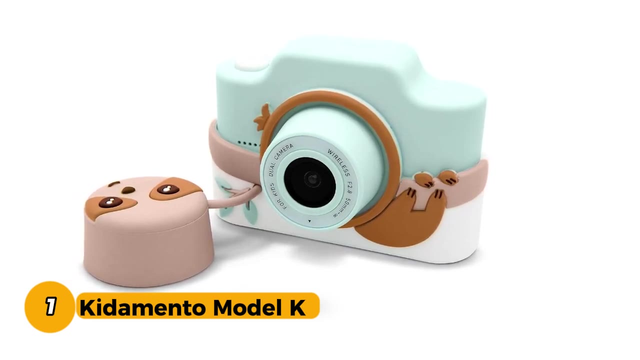 to remember that this camera is designed for kids and the focus is on fun and exploration rather than professional-grade photography. Number 1. Kidimento Model K. Give your child the gift of creativity and fun with the Kidimento Model K Zippy the Sloth, This kid's digital camera. 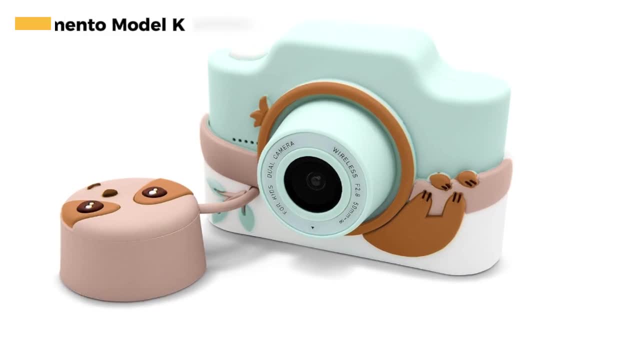 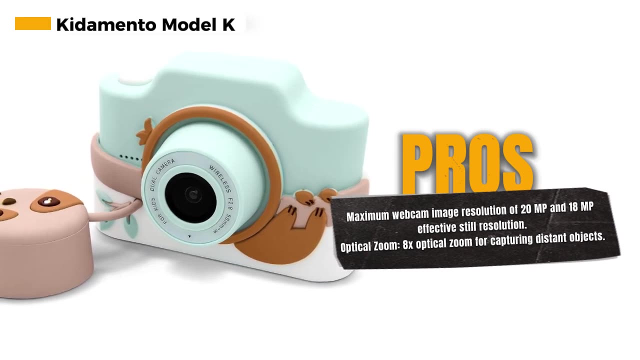 and video camera is a great way to enjoy the fun and adventure of the kids. The camera is a great is designed with your little one in mind, providing a fantastic introduction to the world of photography and videography. The Kidimento Model K is not just a toy but a fully functional. 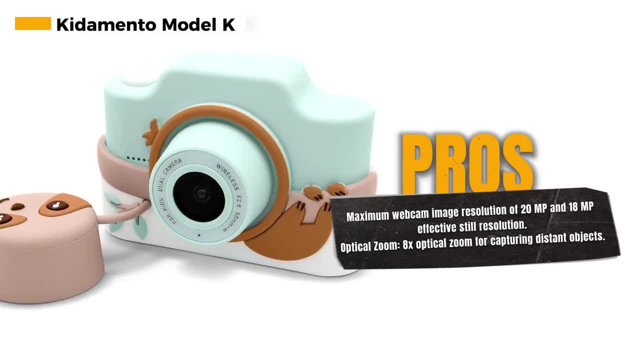 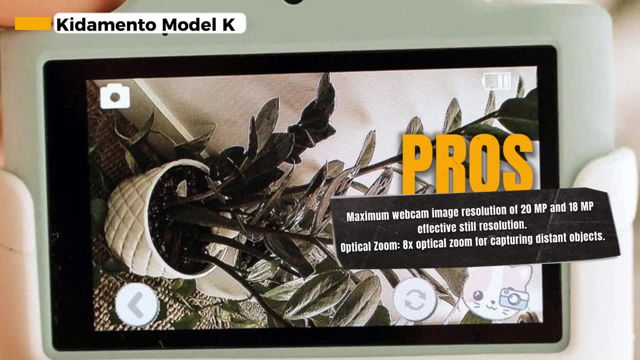 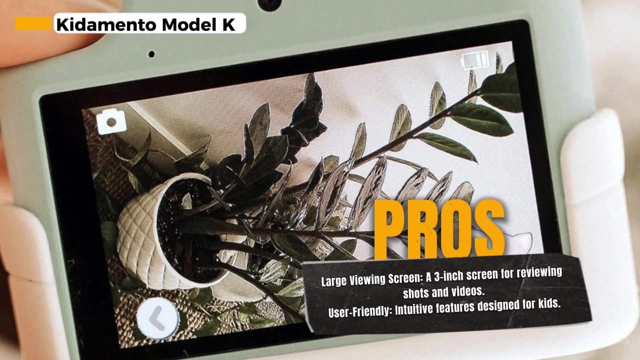 camera with a touchscreen, soft silicone casing, detachable lens cap and even a 32GB memory card included. It's the perfect starter kit for your budding young photographer. Boasting a maximum webcam image resolution of 20MP, this camera captures excellent video and video capture. 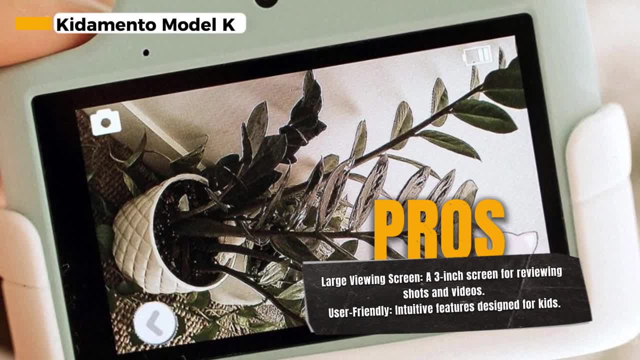 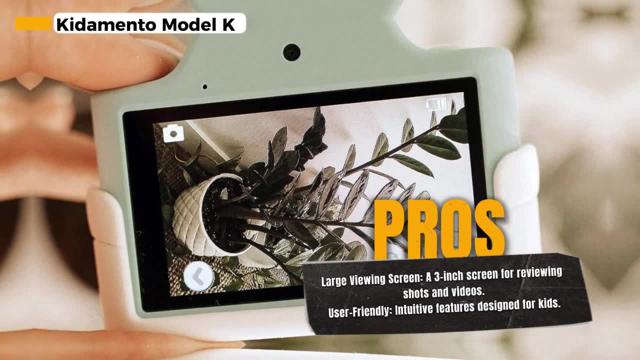 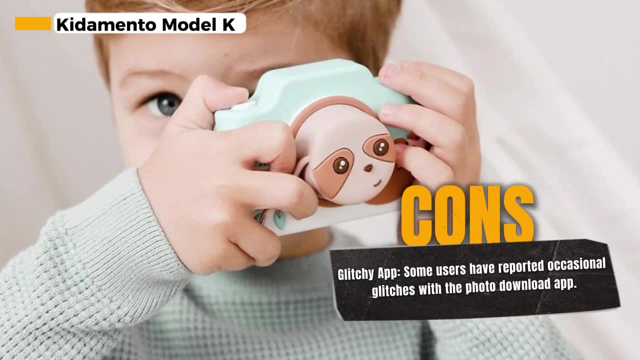 photo quality, ensuring that your child's memories are preserved with clarity and precision. The 18MP effective still resolution is impressive for a camera in this category. The 8X optical zoom opens up exciting possibilities for your child to explore and capture distant objects, making 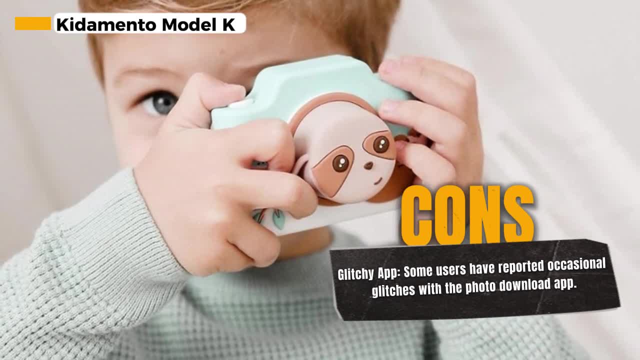 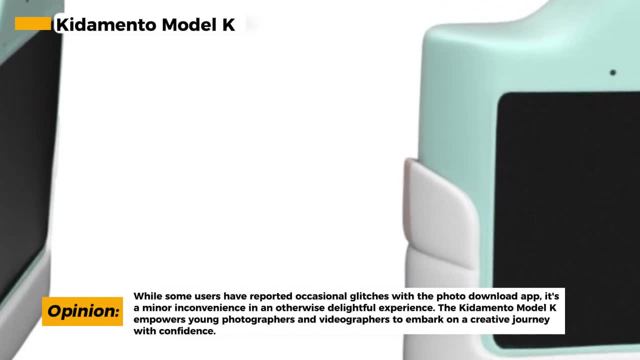 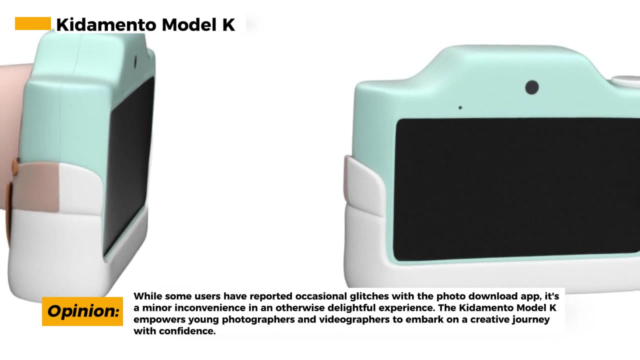 every adventure a visual treat. The large 3-inch viewing screen is perfect for kids to review their shots and videos. It's easy to use and the intuitive features make it a perfect camera for children to navigate, allowing them to express their creativity with confidence. However,